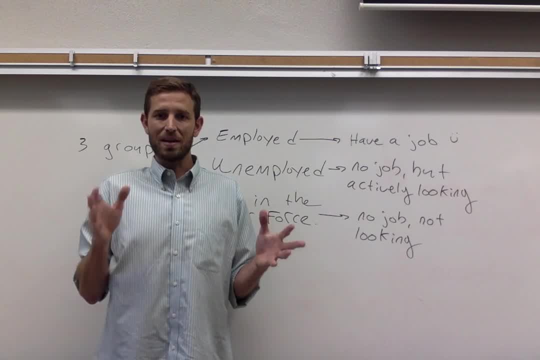 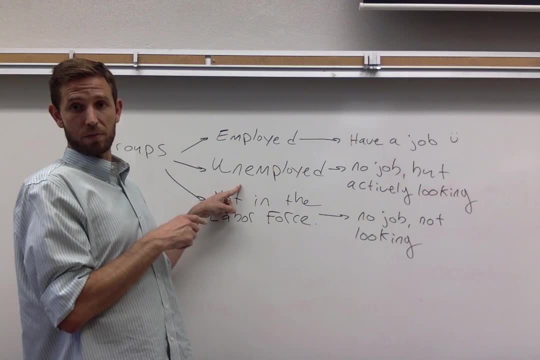 have a job, And so, as I said before, we'd get misleading numbers if we were to count them as being unemployed. So, as a consequence, to fit this definition here of being unemployed, you've got to meet both those criteria: No job and looking. 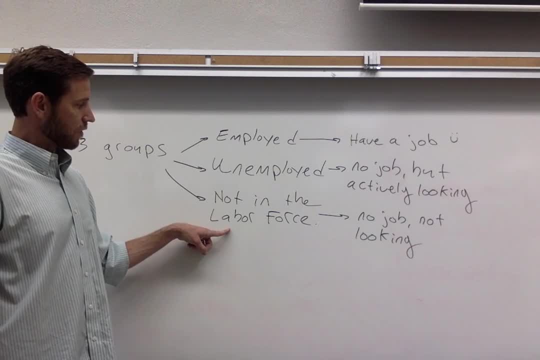 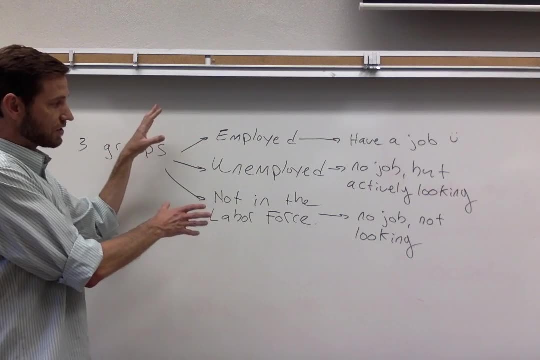 The third category is to be categorized as unemployed, And so here's: the first category of people is the one you see here, and that's folks that are not in the labor force, neither employed nor unemployed. all right, so these definitions, these three categories that all eligible folks are going to fit into, are really 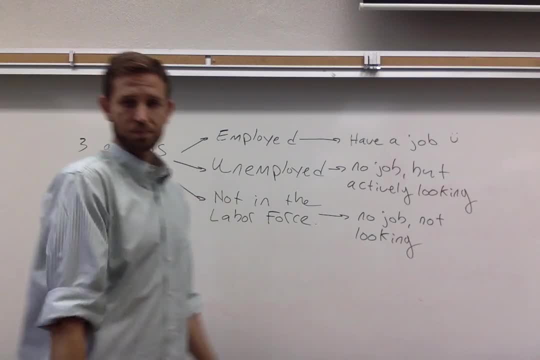 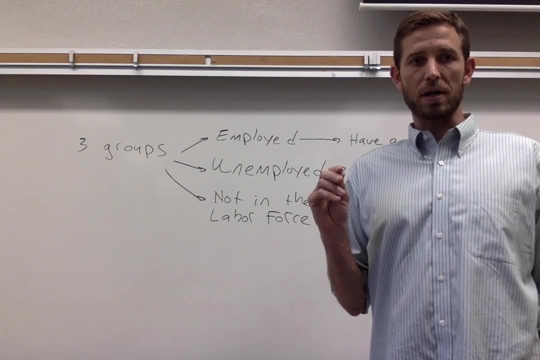 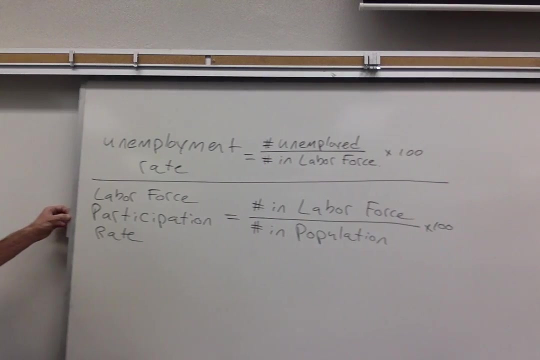 important when you encounter any sort of calculation. all right, as I said a moment ago, there are two key statistics that you need for labor market purposes. right, and I'm going to pull the board over this way to show you the two that you ought to know about. 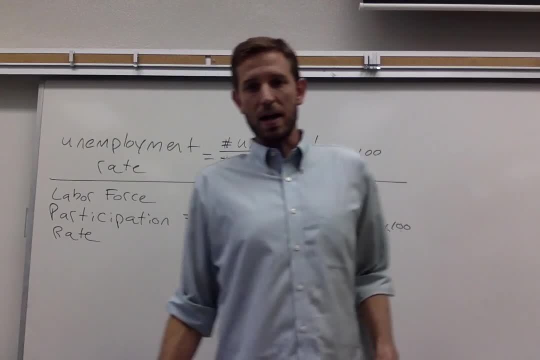 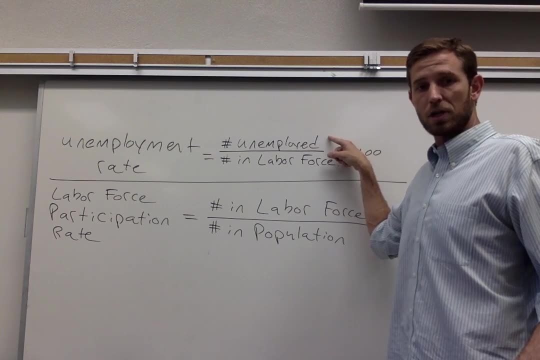 all right. first is one that you've likely heard of before, that is, the unemployment rate, and so this is a straightforward calculation. you just take the number of people out there in the economy or a country that are unemployed, and then you'll divide it by the total number of people in the labor. 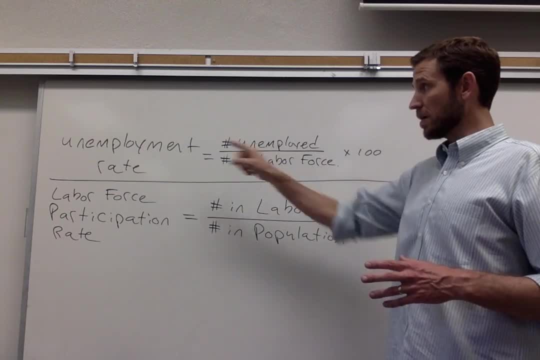 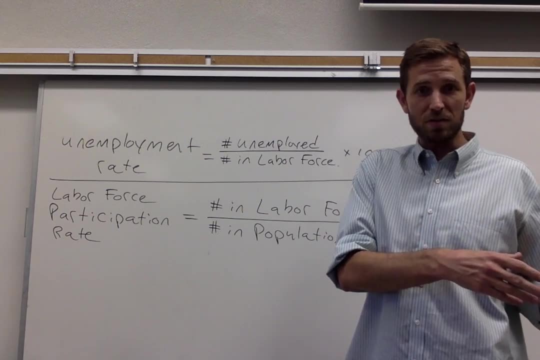 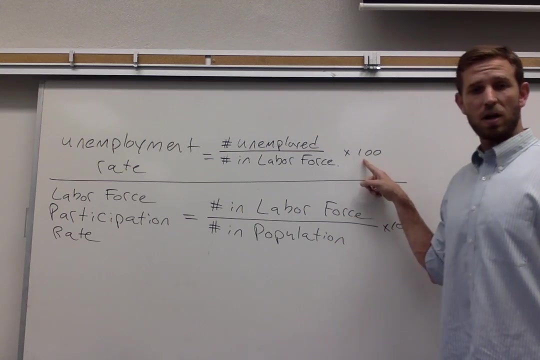 force. right, and so significantly. with unemployment rate calculations, we're leaving out folks that are not in the labor force, right again, those people who are full-time students or retired people or just not in the labor force for whatever reason. right, you want to multiply it by 100 as well, so that you can express that as a percent rather than as a decimal. so 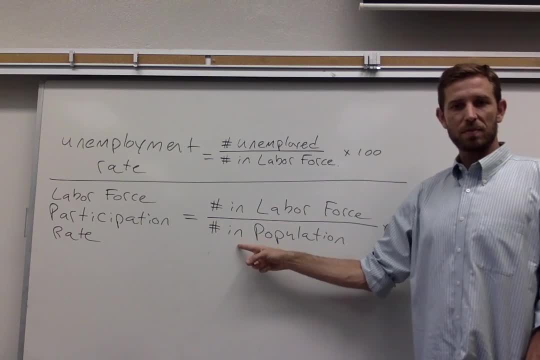 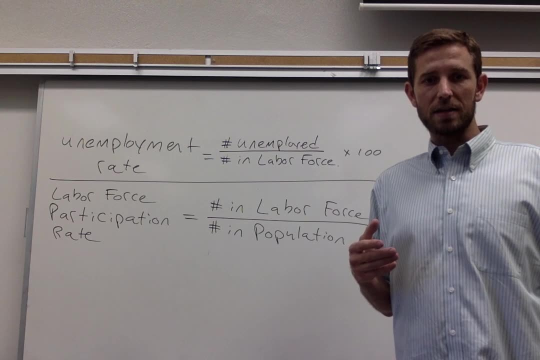 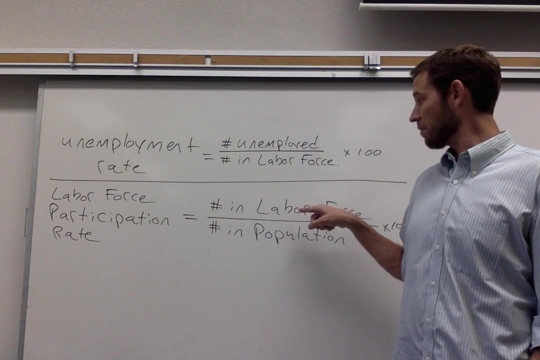 that's one important statistic. another one that you ought to know about is something called the labor force participation rate, and this is a measure of the share of the total population that is actively participating in the labor force, as you might guess. and so the way to calculate this: you just take the number. 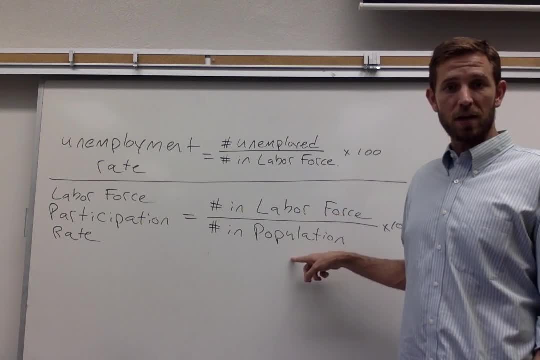 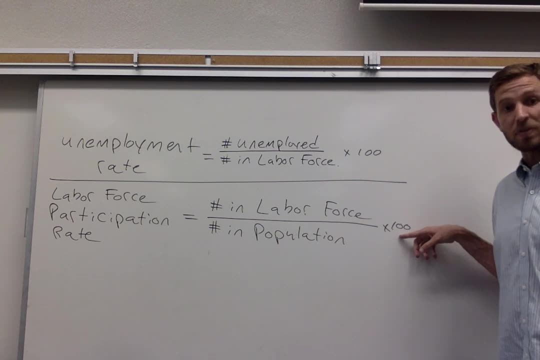 of people who are in the labor force and divide that by the total eligible population. once again, you want to multiply that whole thing by 100 so that you can express it as a percentage, and so the formulas here are straightforward. really, the important thing is understanding who fits into each. 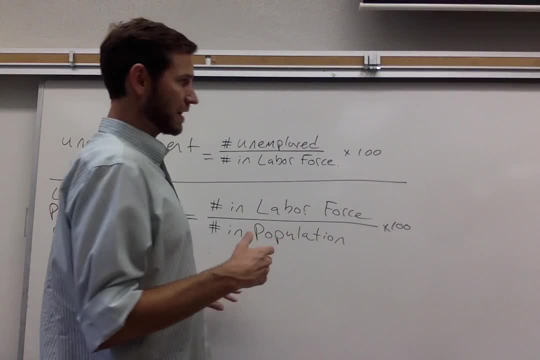 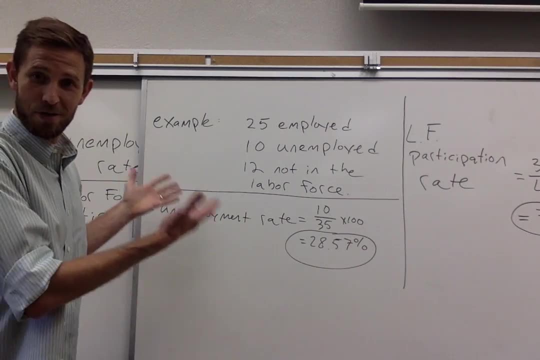 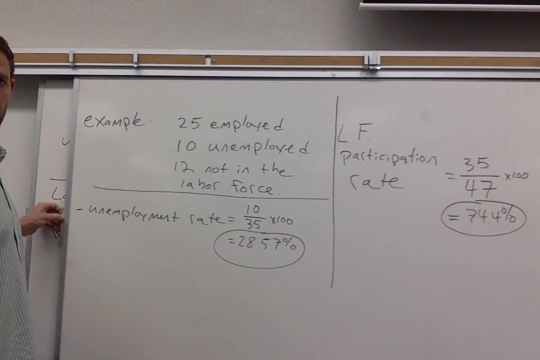 of these categories. all right, last thing that I want to do in our lesson here is to give you guys a quick example. so on board number three, here I've got some numbers that we can work with. alright, so it's likely you're going to encounter a problem where you're given. 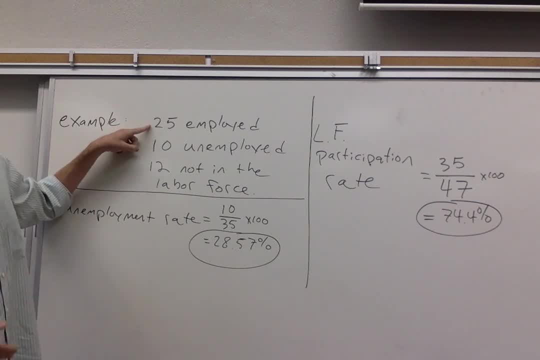 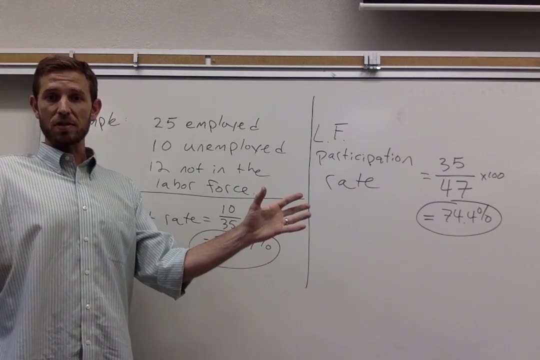 information similar to what you see on the board right. so some estimate of the number of people who are employed. again, it might be presented like this: just people employed, or it could be some full-time and some part-time workers. you just take all those people, lump them together, find the total number of people. 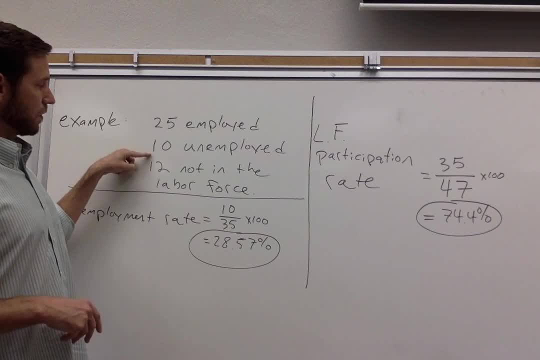 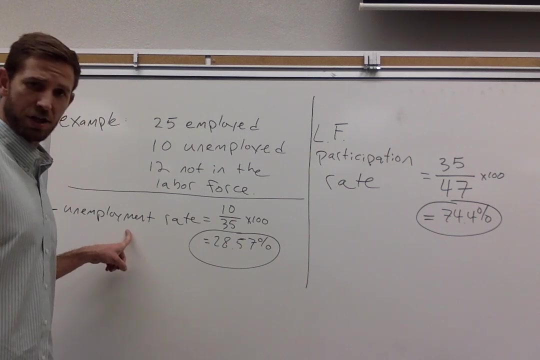 employed. in this case, we've got 25- 10 people in this problem who are unemployed, and then we also have another 12 people who are not in the labor force. right, based on a set up like this, we can calculate those two statistics that I showed you just a moment ago. so let's do that really quickly. but first, here we 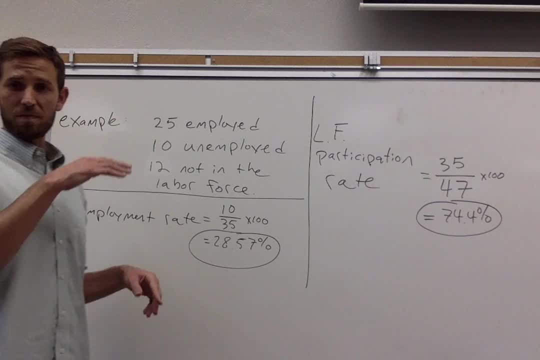 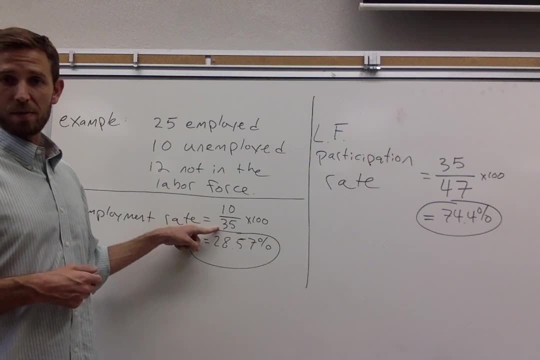 want to calculate the unemployment rate, again that's the number of people who are unemployed, and take that information directly from the problem set up- never 10 of them- and then we want to divide it by the labor force, which, again the a labor force is the sum of employed and unemployed people, right? 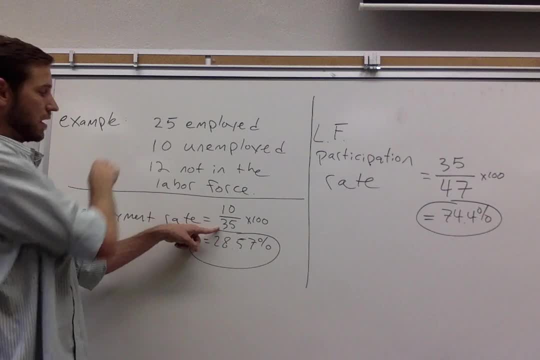 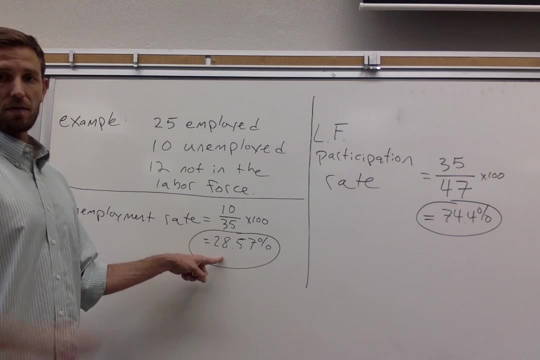 So that 35 comes from summing that 10 and that 25. right there, right, Don't forget to multiply it by 100.. Once you get that, you're going to see the result here that the unemployment rate for an economy like this would be 28.57%. 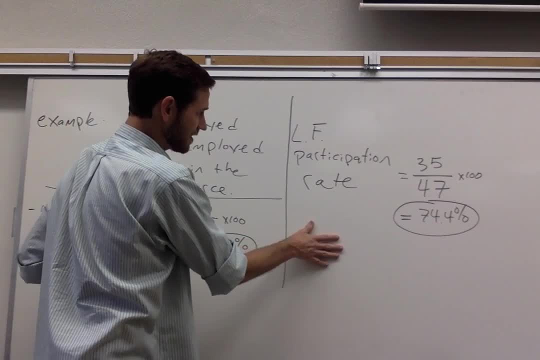 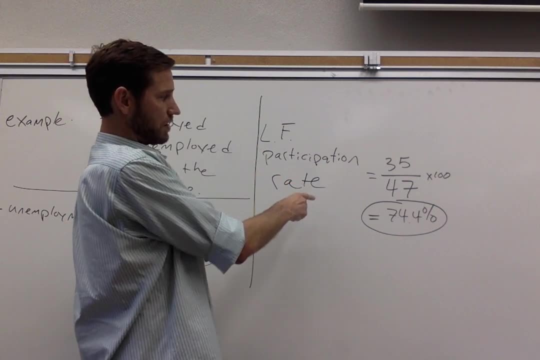 That's bad, All right, That doesn't show the whole story. You also might be interested in looking at labor force participation rate as well. All right, and so the way to do this, you're going to divide the number of people who are participating in the labor force. 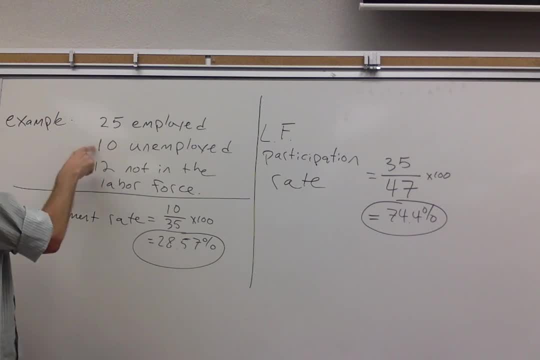 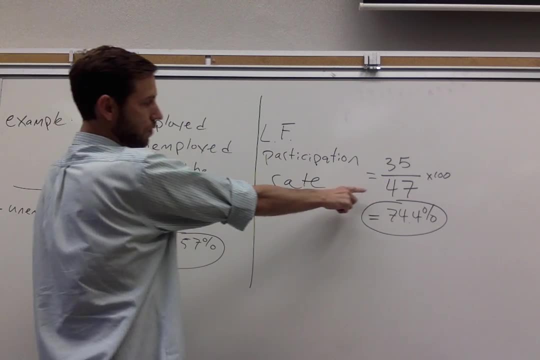 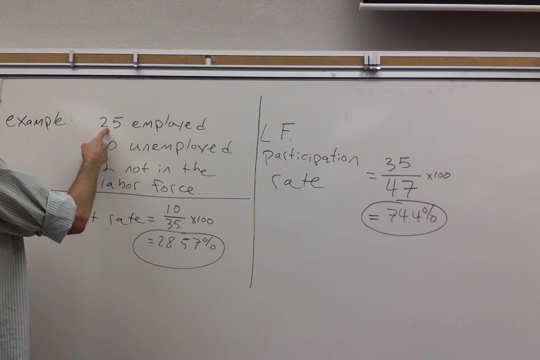 That's 35.. The sum again of 25 and 10 employed and unemployed people And you want to divide that into the number of people who are in the population right, So that 47 here comes from summing 25 employed people.